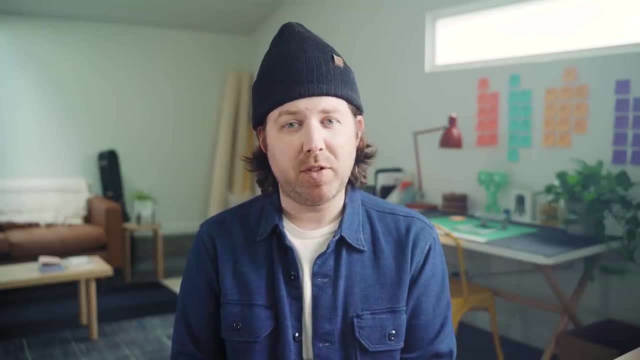 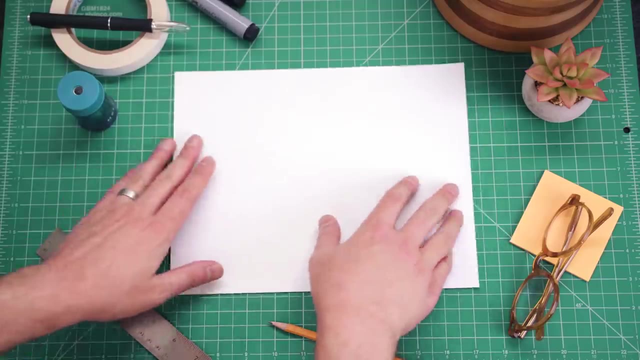 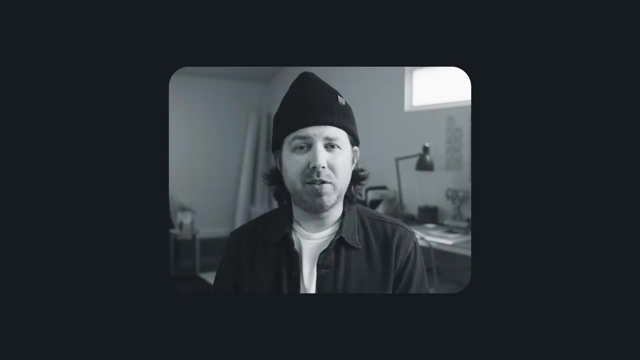 it in your own work, then check out my course Color for Creatives. We cover everything you'd ever want to know about color theory. As for the rest of you, here comes tip number one: Color harmonies. People love to ask: hey, Greg, where do I even start with color? It's a good. 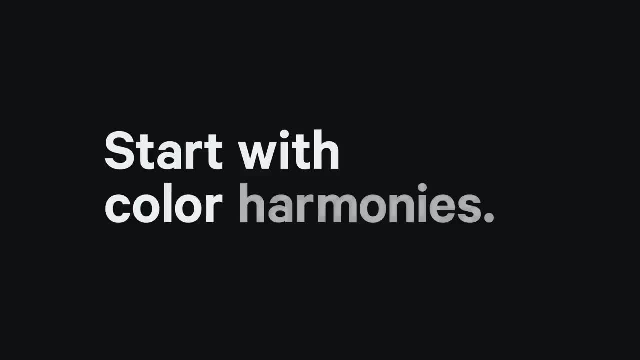 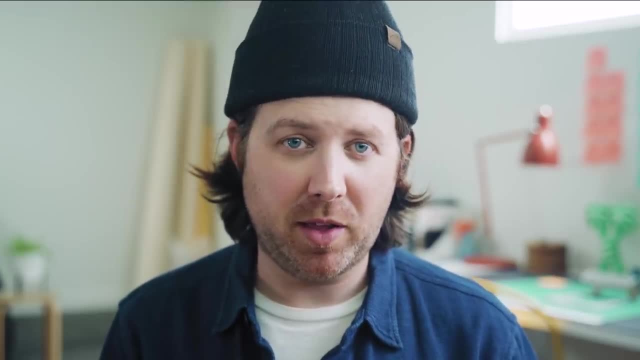 question and my answer to them is always: start with color harmonies. Color harmonies are historically used to create color harmonies and they're often used to create color harmonies- historically proven, science-backed techniques to pair colors together in visually pleasing ways. 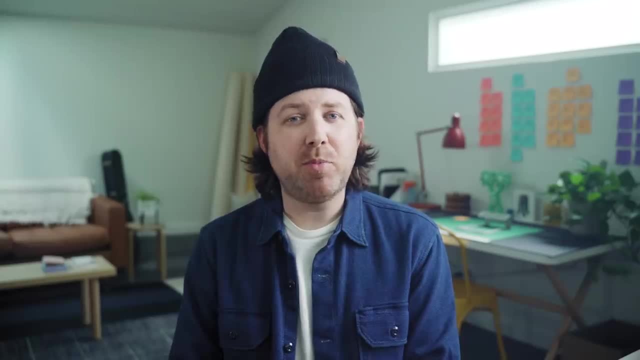 which sounds way more complicated than it actually is. In fact, you probably already know some color harmony terms like monochromatic, complementary and analogous, and all they do is describe the relationship between where these colors are on the color wheel. Some apps even have color harmony. 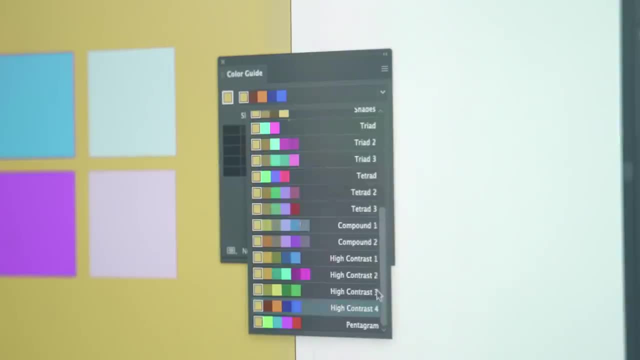 tools built right into them, like Adobe Illustrator's Color Guide and Procreate's Color Harmony Tool. Okay, let's say, you're a color artist and you're a color artist, and you're a color artist and you're a color artist. 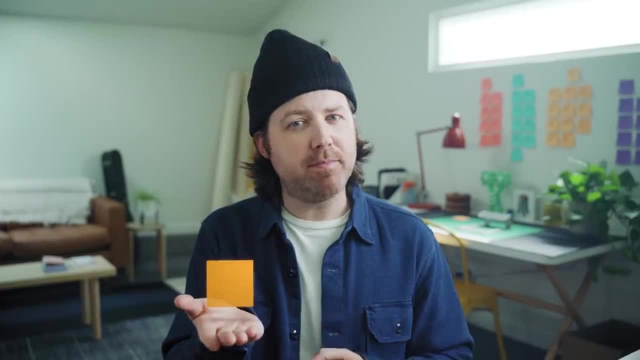 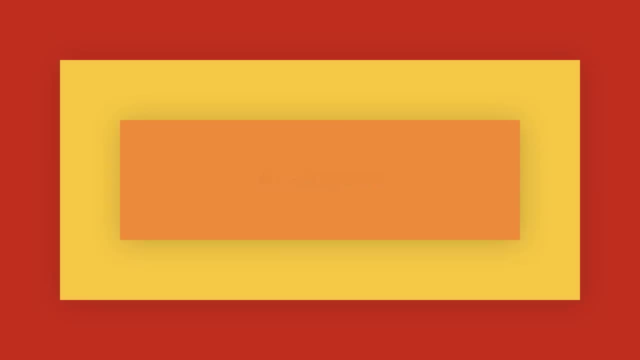 let's say you love this orange but you're not quite sure what to pair with it. Color harmonies to the rescue. You can play with different harmonies, see what you like and then adjust to taste. In this case, I'm feeling like split complementary is the move. So if you're not quite sure where to, 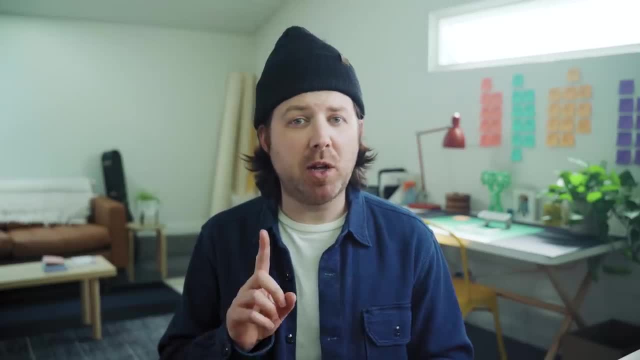 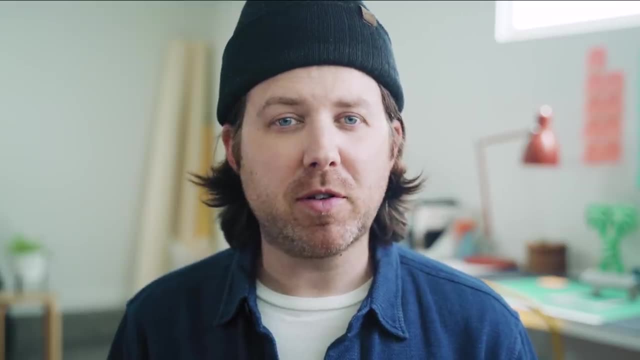 start, consider a color harmony. All you need to do is find one color that you like and then let science do the rest. Tip number two: neutral colors. Neutral colors are like the supporting cast for your lead colors. They can be warm, they can be dark, they can be dark, they can be dark, they can be. 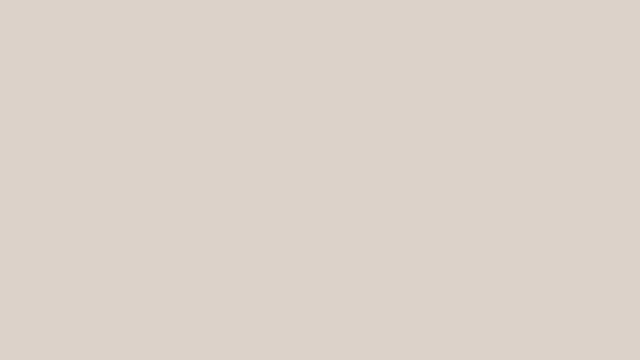 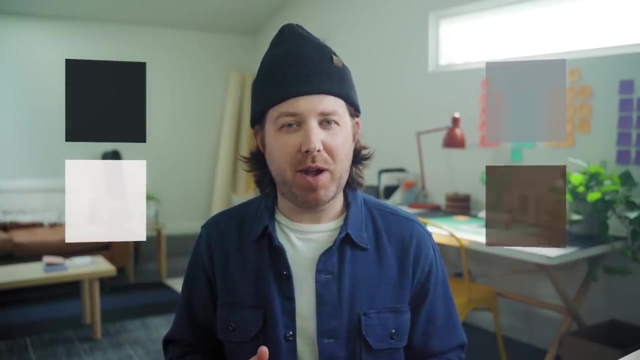 warm, cool, light or dark, and they tend to recede into the background, leaving room for your big, bold color choices. The most common neutral colors are blacks, whites, grays and browns, and their most notable trait is that you can't really tell what the underlying color is, hence the term. 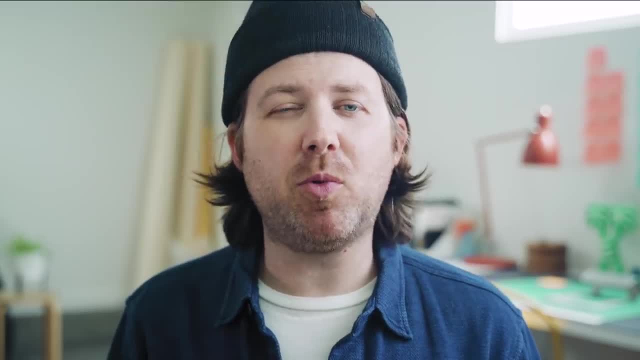 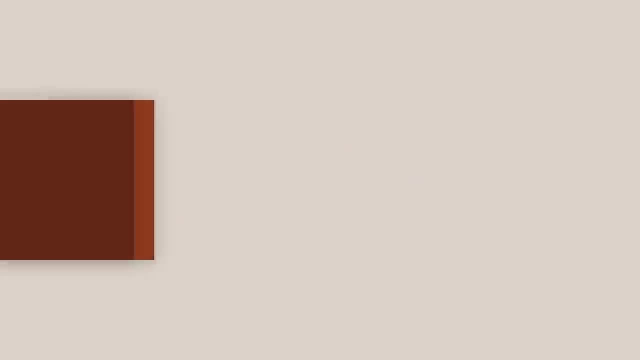 neutral. The benefit of using neutrals is that they offer visual relief from your primary colors and, by contrast, they make those colors stand out that much more. Think of them like negative space, but for color, And you probably need more than you think. 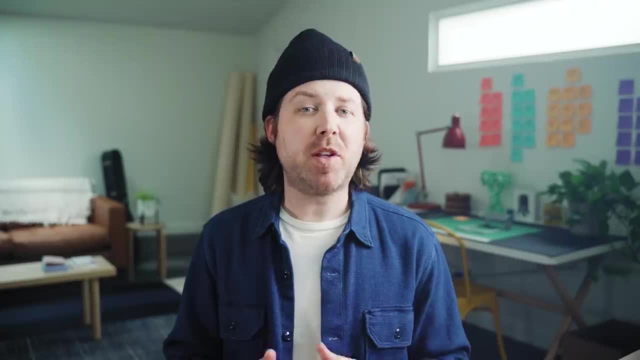 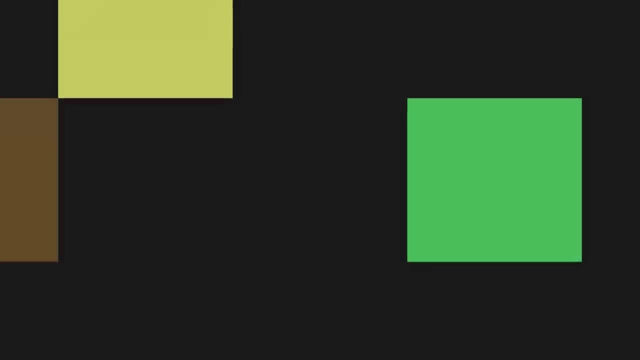 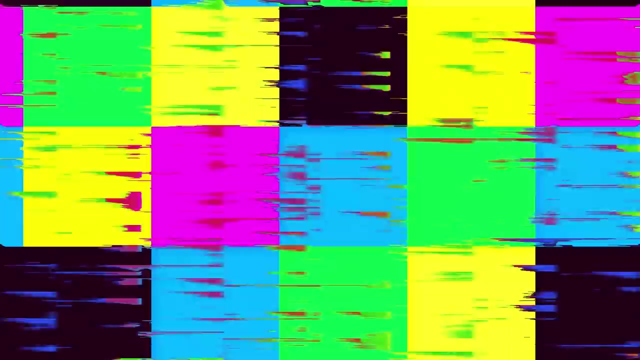 Tip number three: less is more. The most common color mistake I see is overuse, and the second most common is oversaturation. The more colors you have to work with, the more difficult it becomes to get them to work together. If they're all bold, bright and vibrant, it can become a real mess, And I get 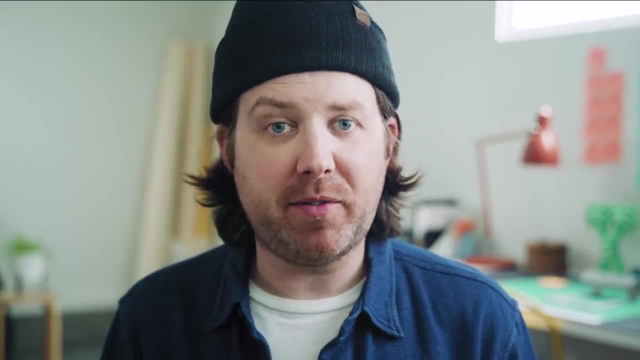 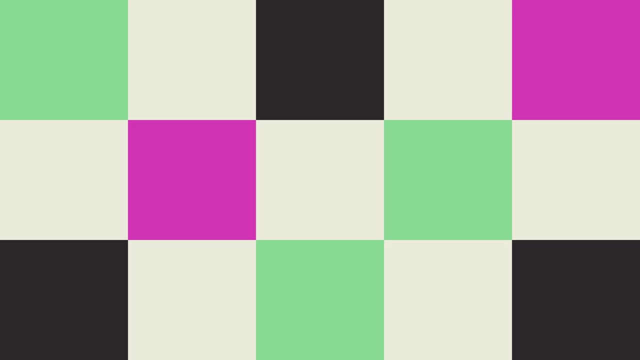 it. I love using all the colors. We've got this endless supply of digital crayons. Why not use the whole box And you know what We totally should, Just maybe not all at the same time and on the same project. Think about when you cook, You don't use all the spices from the rack. 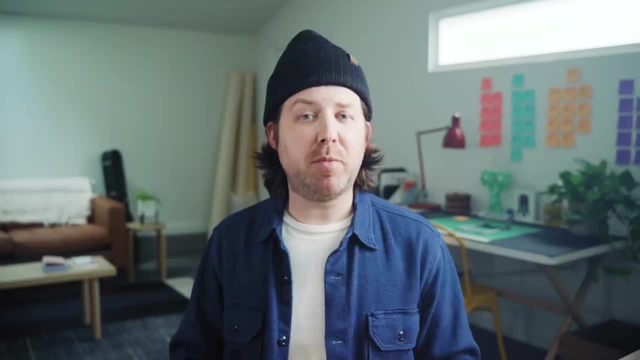 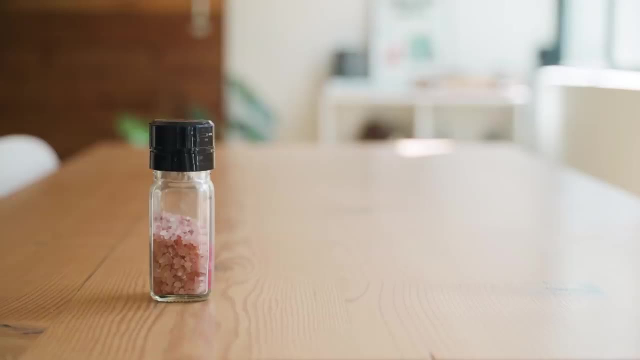 Just the ones that you know will make the dish taste really good. So before you go wild with color, think about the mood you want to create, The visual flavor, so to speak, Because maybe all you need is some salt, pepper and smoked paprika. Start with two colors, then maybe two neutrals. 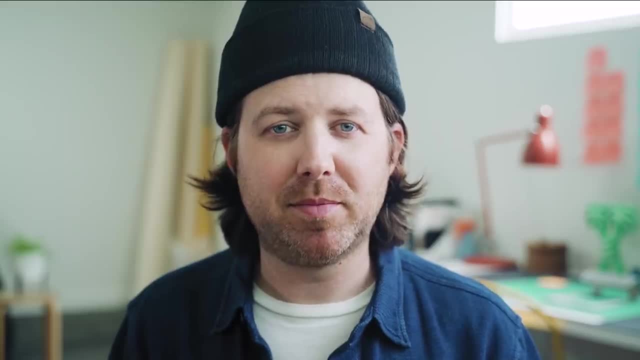 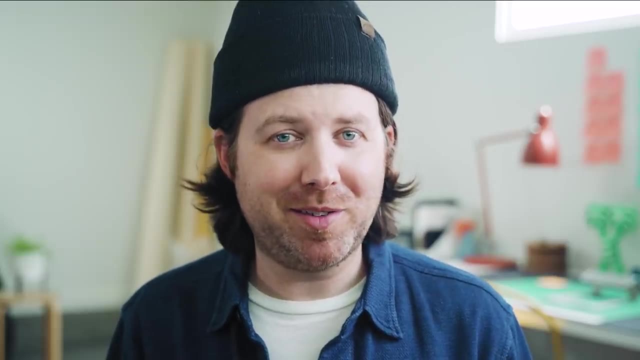 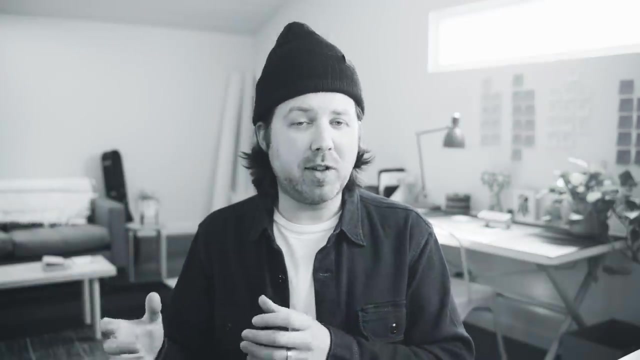 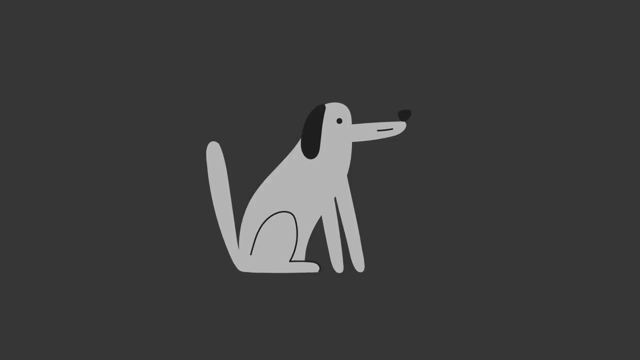 See how that goes. You can always add more later. Tip number four: Contrast. Okay, want to know the real secret about using color well, Contrast. It sounds counterintuitive, but the way your image looks in grayscale will determine how good it looks in full color. The value of a color as in its lightness is almost more important than 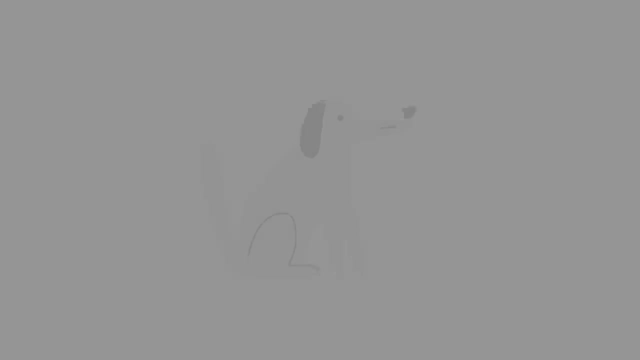 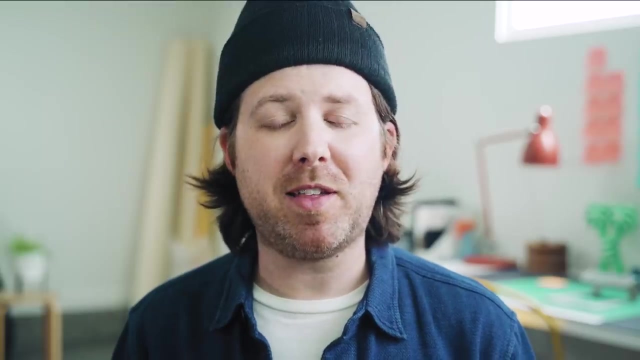 the color itself, Because without enough light and dark contrast, your image will be lost And at that point the colors don't really matter. So if you're using a color that's light, it's not going to really matter. Low contrast is a great way to frustrate and alienate people. 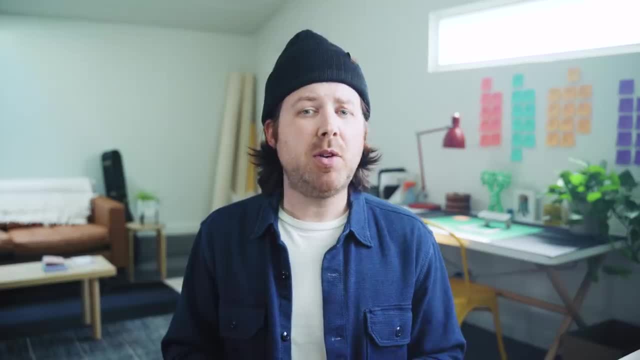 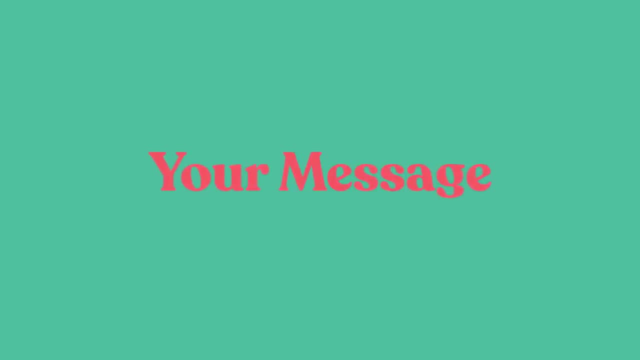 from your work, especially when typography is involved. Not only will low contrast make something difficult to read, see or experience, but it can render your message illegible or even invisible to people with color blindness, Which is why having strong contrast, especially with type 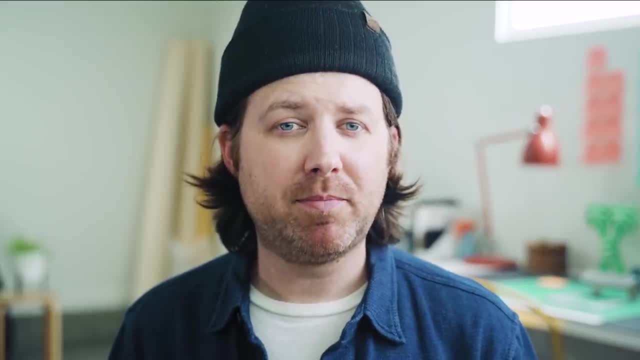 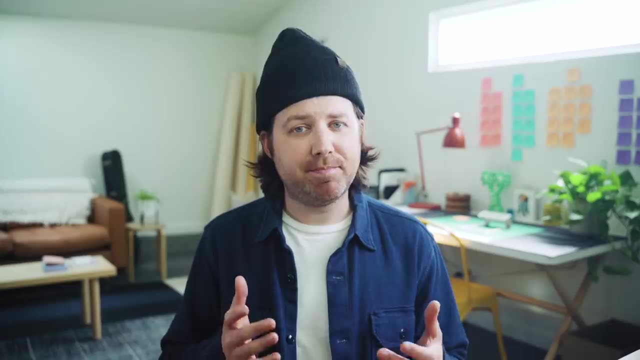 is crucial to accessible design. My general rule of thumb: If it works in grayscale, it'll work in color. So get in the habit of checking your color values. Easiest way to do that: Convert your work to grayscale. And if you're using photoshop, 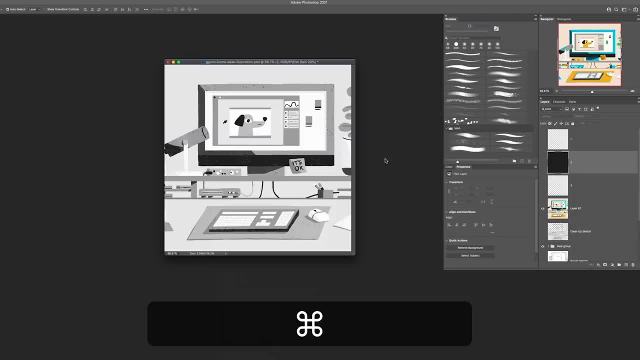 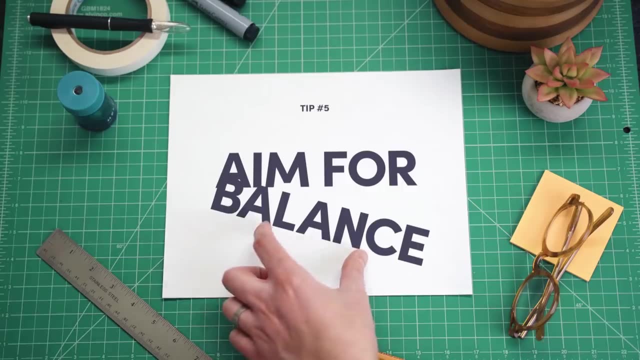 set your proof mode to grayscale and then tap command y or control y to toggle a black and white preview. And big ups to Marco Bucci for that clever time-saving tip. Tip number five: Aim for balance. Working with color is a lot like playing an instrument. You want things to just. 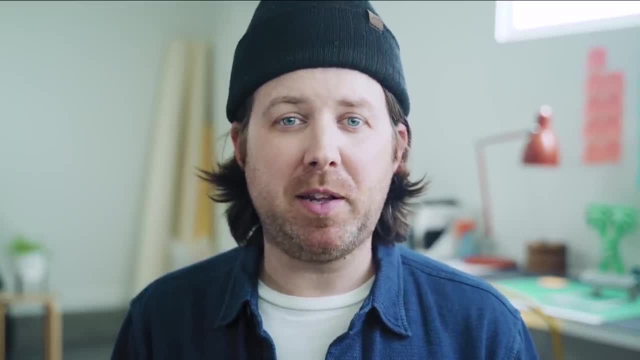 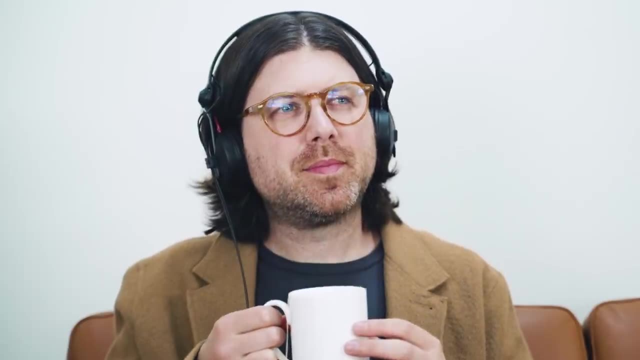 kind of naturally flow. You don't want to play the same chord, at the same speed, at the same volume throughout the whole song. It'll get really boring. And this is coming from a guy who loves metal. Imagine your colors are musical notes. You want to make sure there's a nice range of values, of hues and of saturation. It's all about the relationships between colors. You can't have light without dark and everything else in between. Not every color needs to be a star either. Let one or two take the lead. 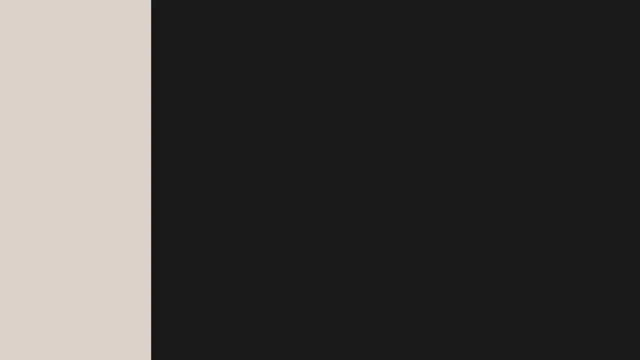 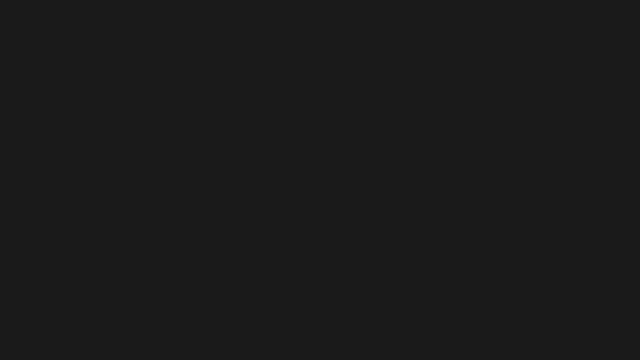 And then have the rest. keep rhythm. Remember neutral colors. They're the rhythm section. Also, think about how much of each color you're using. The 60-30-10 rule is a great place to start. In this case, we'd use our primary 60% of the time. 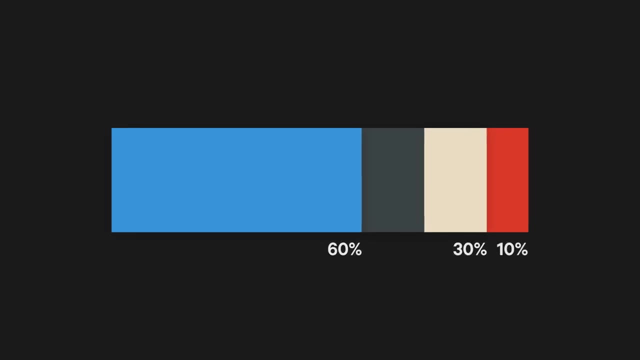 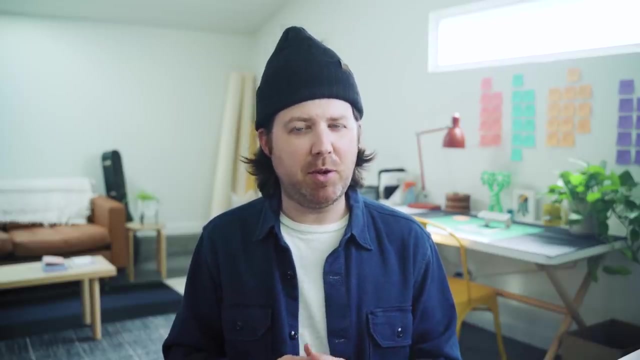 our neutrals 30% and save our accent color for the very last 10%. Striking the right balance with colors is tough. It's like the sum of the first four tips. You want harmonious colors, room to breathe and plenty of contrast. 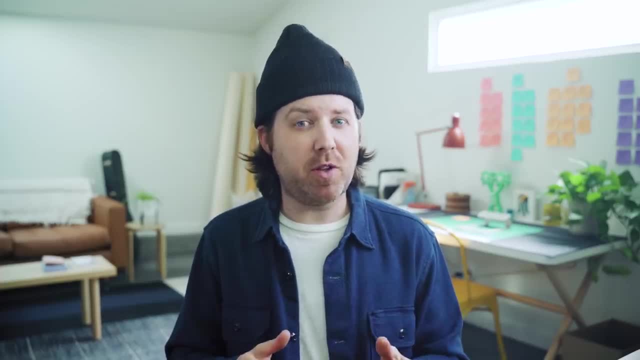 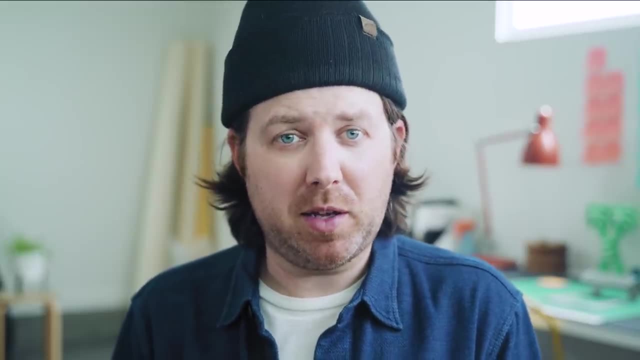 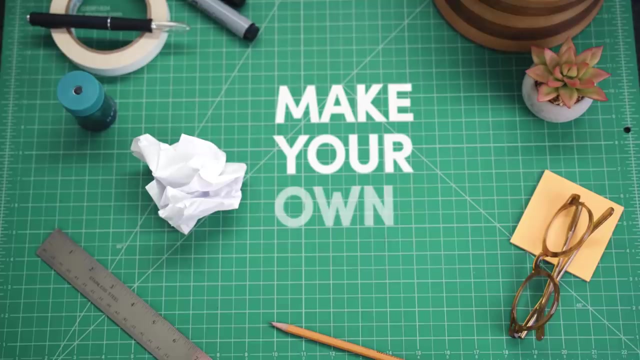 Bonus tip Now, despite what you might hear strangers on YouTube tell you, there are no hard and fast rules for using color. There are best practices and methods that work really well, like color harmonies, But ultimately it's a subjective experience. So my last tip for you is this: Make your own rules. It's your work, You can. 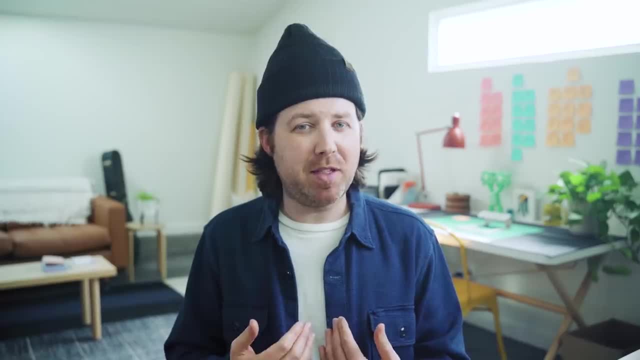 use whatever colors you want. however, you want My two cents, though. Just be consistent in how you use them. That way, you don't have to worry about what colors you're using. You're going to get the best results. That way, we, the viewer, understand what the rules are and we have a much 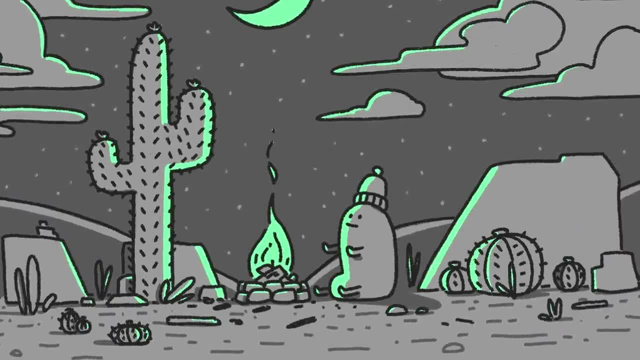 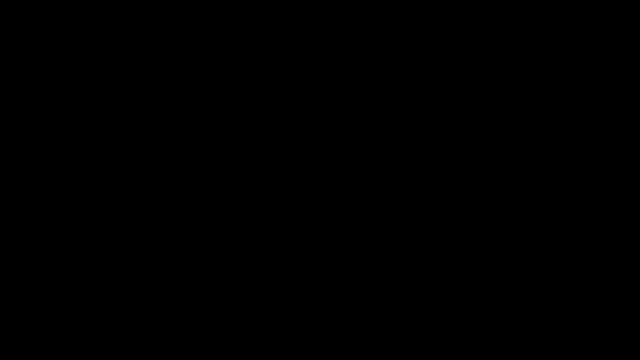 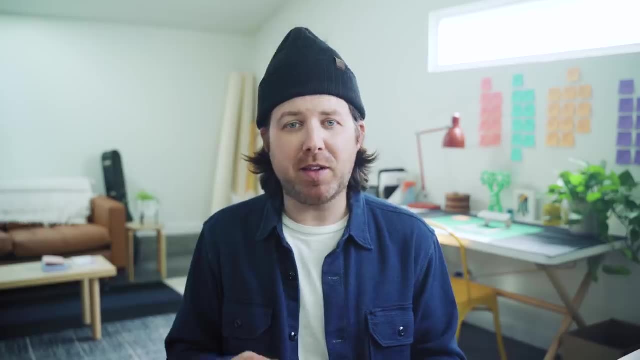 better experience. So if you want to make your highlights green and your shadow colors orange, go for it. Just make sure that all your shadows and highlights follow suit. Like I said up front, working with color can be really frustrating, which is why understanding concepts like color harmonies and contrast is so important. 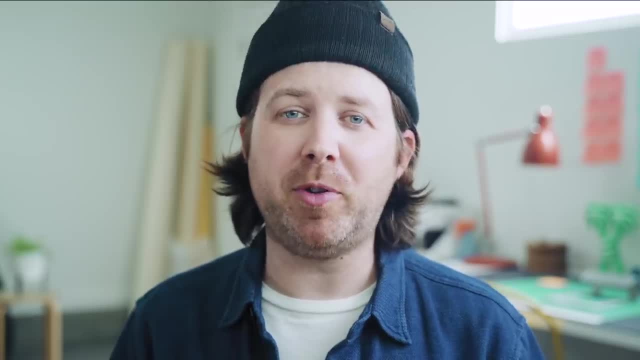 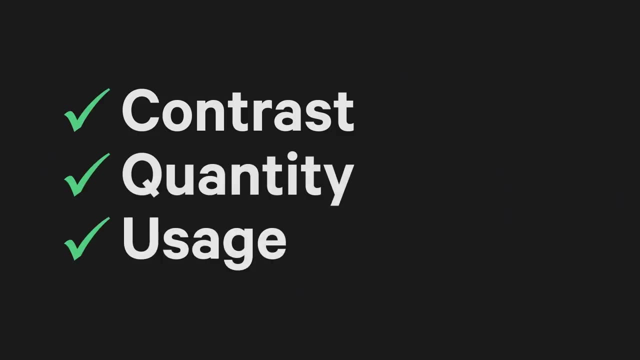 I gave you six tips in this video, but if there's one thing I hope you take away, it's the concept of balance. Striking the right balance between contrast, quantity and color usage is what will make the biggest difference in your work. So remember, color is a lot like music. 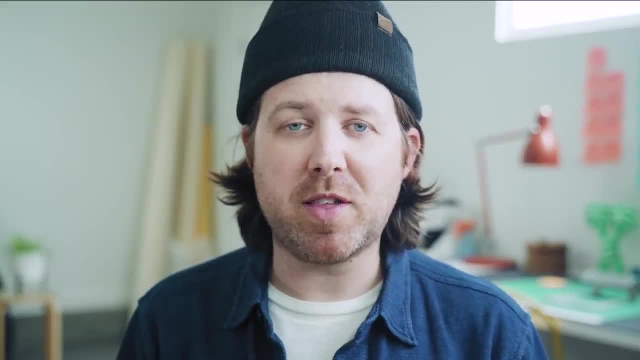 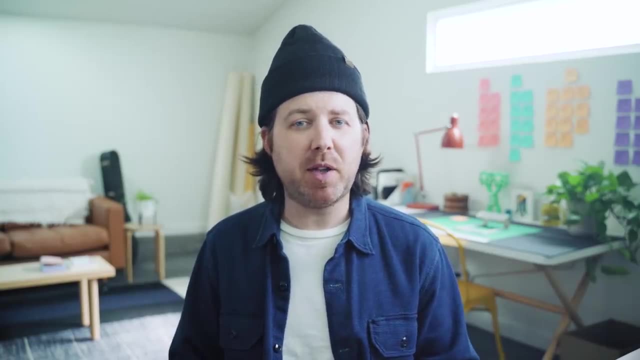 Each note has its place, and the quiet moments are just as important as the loud ones. What's your favorite color tip? Share it in the comments below, and let's use the collective power of the intranet to make a color tip megathread.